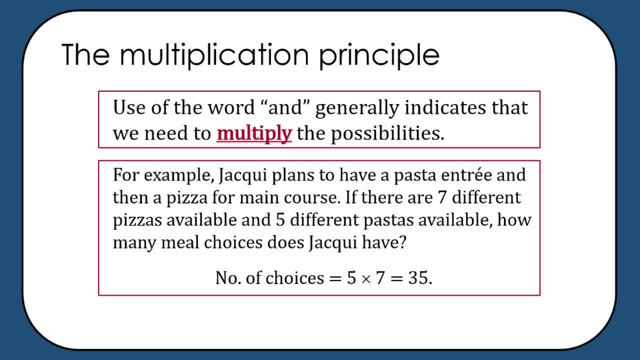 So because she's going to have both a pizza and a pasta, we're going to multiply together the number of options of pizza and number of options of pasta to get 35 total choices. And really this is about if you were to think about drawing a tree diagram here of what might happen. so the first stage of the tree diagram would be her entree choices, her pasta choices and she's got five different pasta choices. so there'd be five branches at the first stage of the tree diagram. 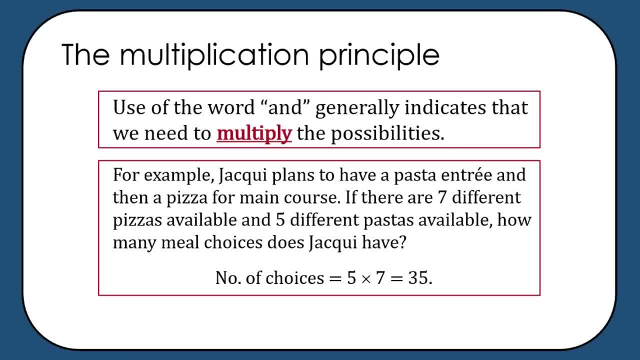 And then for each of those different entree choices, she then has a choice of seven different pasta choices. So you would then from each of those initial five branches draw a further seven branches, branching out, And the result would be that there'd be 35 choices. 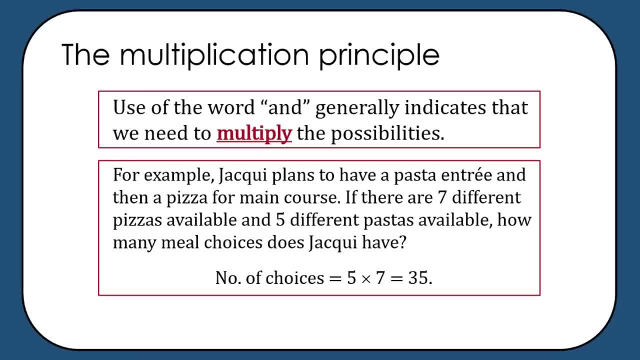 So there'd be 35 different branches at the end of the day. So you know, she could have the bolognese followed by the Hawaiian pizza, or she could have the bolognese followed by the capricciosa pizza, or she could have the carbonara followed by the margherita pizza. 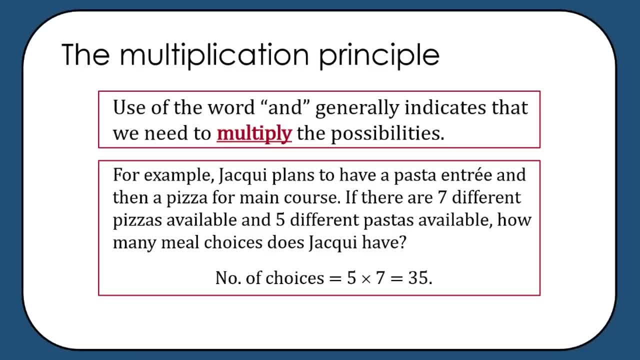 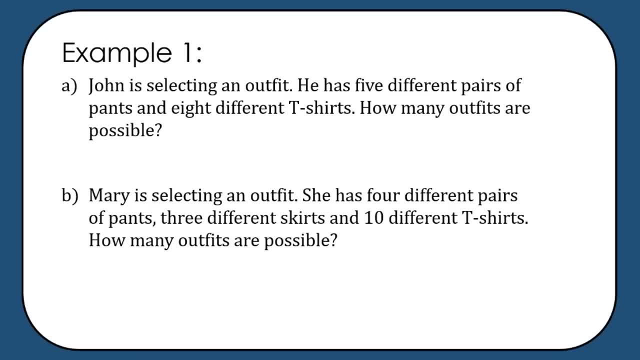 And so there'd be all the 35 different options of what she could have. So we're generally looking at: OR indicates addition and indicates multiplication. Let's have a look at some examples. So Mary is selecting an outfit. He has five different pairs of pants and eight different t-shirts. 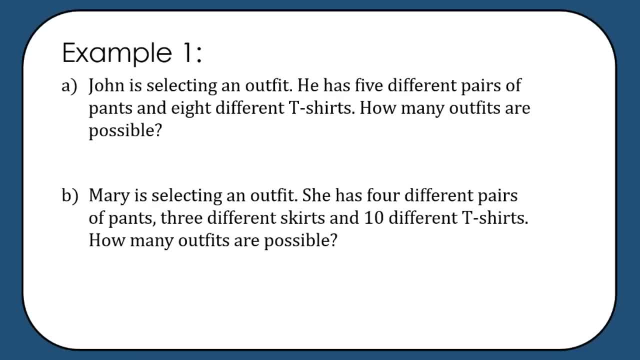 How many outfits are possible. So he's going to wear pants and a t-shirt, So we're going to need to multiply together the options here. So he has five pairs of pants and eight different t-shirts, So altogether there is 40 different outfit combinations that he could wear. 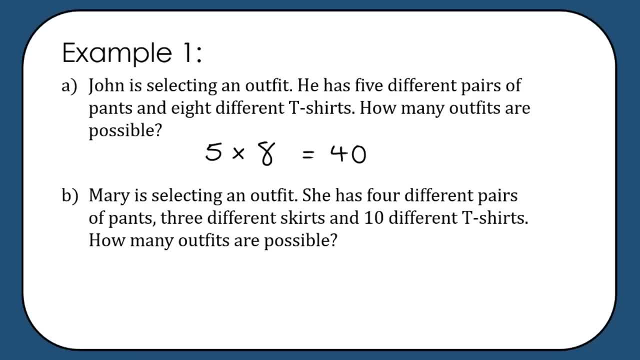 Mary, on the other hand, is selecting an outfit, And she has four different pairs of pants, three different skirts and ten different t-shirts. So, whilst up here with John, he was going to wear pants and a t-shirt, Mary's going to wear pants or a skirt. 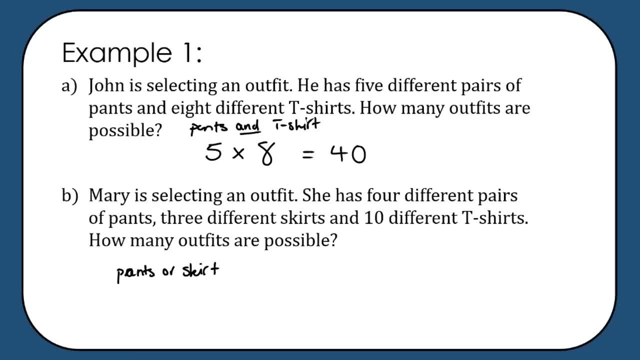 So that's going to be her first choice, And then she's also going to wear a t-shirt. So there are four different pairs of pants and three different skirts. So all means we're going to add. She's got seven different options for her bottom half. 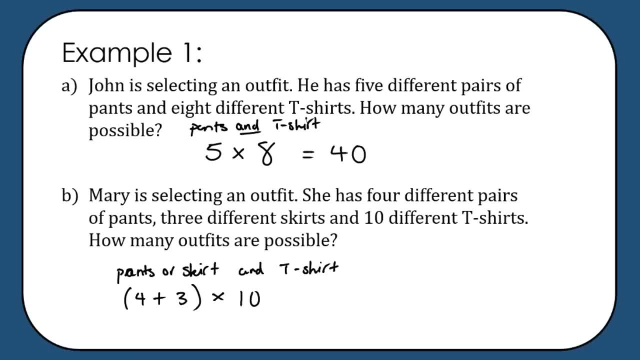 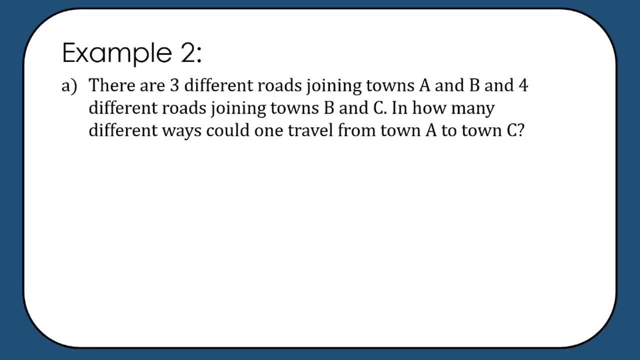 And she's also going to wear a t-shirt, So there are ten different t-shirts she could wear, So seven different bottoms and ten different tops, And so therefore, she has 70 different outfit choices. Okay, so there are three different roads joining towns A and B and four different roads joining towns B and C. 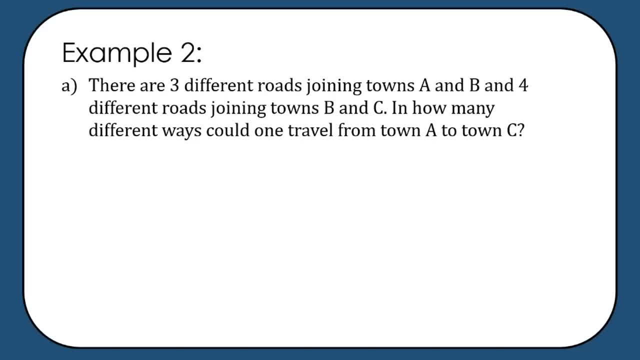 And how many different ways could one travel from town A to town C? Okay, so you're going to go from town A to B and from town B to C, So you need the number of options of getting from A to B, which is three. 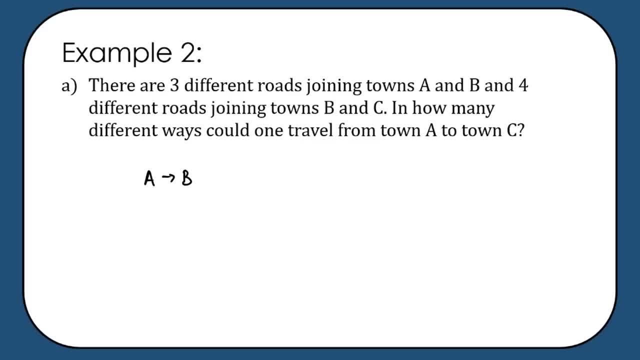 So we're going to go A to B and B to C, So we're going to have three options. So we're going to have three options for this. and indicates that we multiply four options for this. So there's 12 different routes that you could take to get from A to C via B. 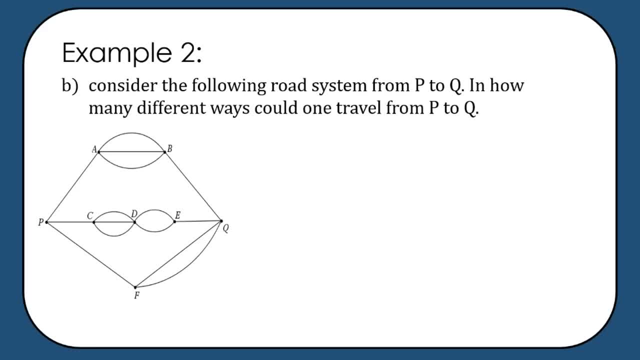 Okay, here we have another road system. In how many different ways could one travel from P to Q? Alright, so there's more options here. So we could go from P to Q going via A and B. So we could go P to A to B to Q. 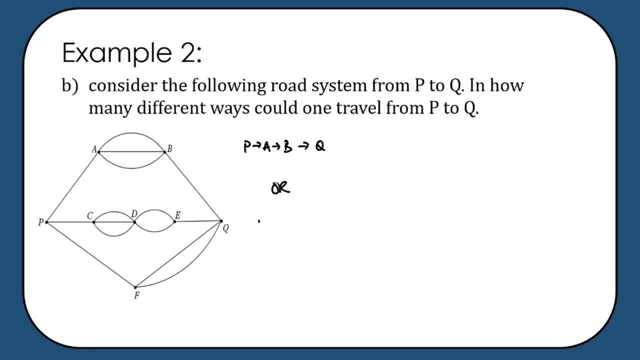 Alright, so there's more options here. Or we could go P to C to D, to E to Q, Or we could go P to F to Q. Okay, so we're going to have if we're travelling from P to A to B to Q. 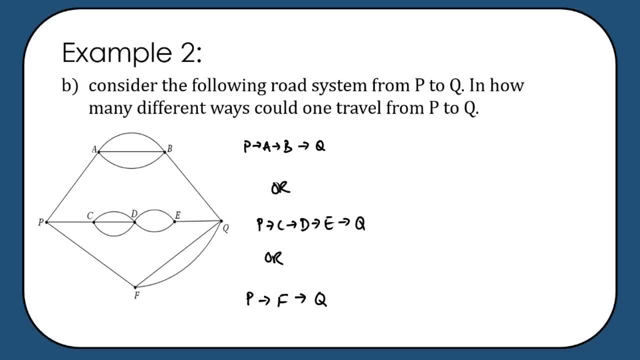 there's only one way to get from P to A, So we need to go from P to A and also then from A to B, and also then from B to Q. So we need to multiply together the options along the journey. So there's only one option: to get from P to A. 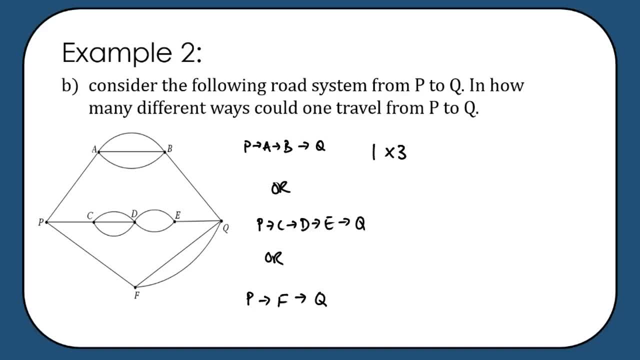 There's three options to get from A to B And then only one option from B to Q, So there's three different ways. we could travel via A, B, P, C, D, E, So P to C, there's only one option. 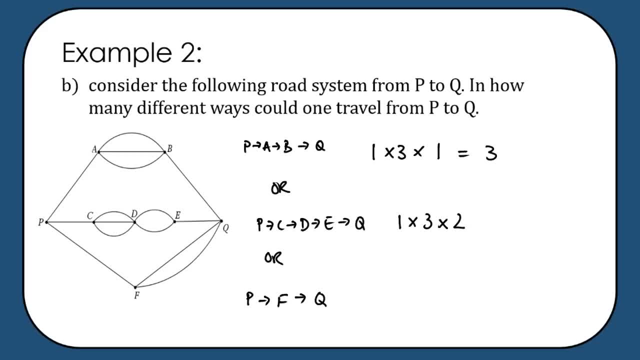 C to D, there's three options. D to E- there's two options, And E to Q- there's one option. So there's six different ways we could travel from P to Q via C to D. So there's six different ways we could travel from P to Q via C to D. 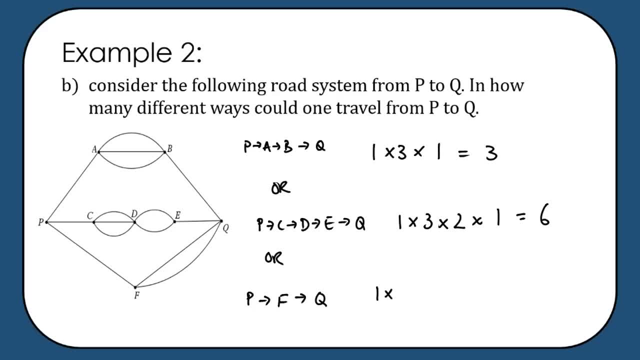 And from P to F. only one option to get from P to F and then two options to get from F to Q. So two different ways. we could go from P to Q via F. So therefore, the total number of total different journeys that could be taken, we've got all here, so we're going to. 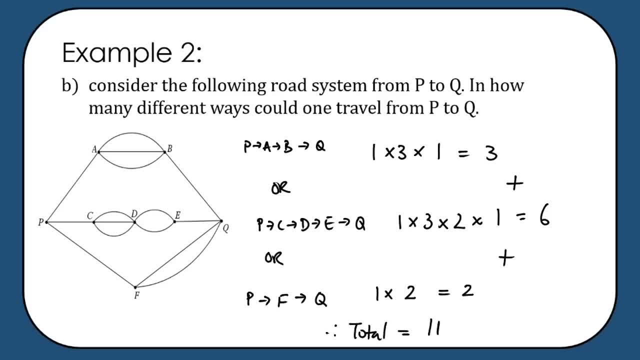 add 3 plus 6 plus 2, so there is 11 different ways. Obviously, in a diagram like this, yes, you could probably count them, but you're starting to think about methods that are going to generalise out to situations with much larger numbers where you know, just simply being able to count it or work it out in that way. 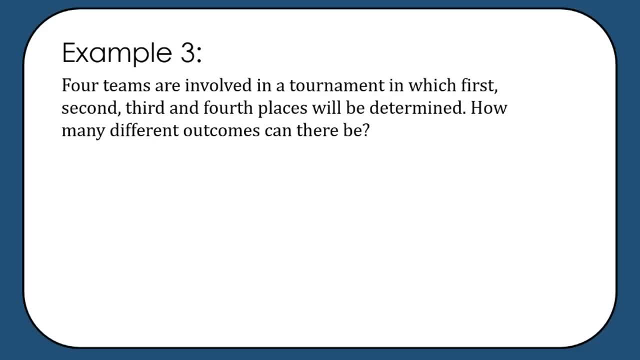 is going to be tedious. Okay, example three: Four teams are involved in a tournament in which first, second, third, fourth, fifth and sixth are involved in a tournament. If the first, second, third, fourth, fifth and sixth are involved in a tournament, 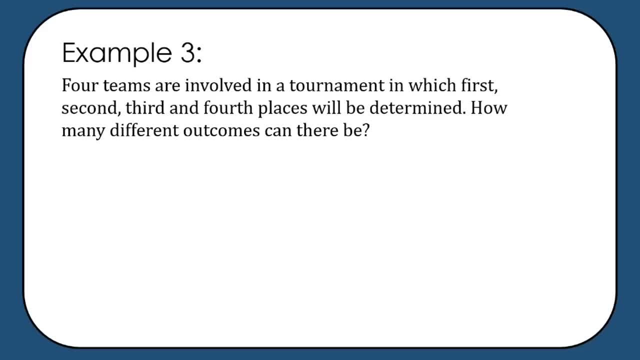 third and fourth places will be determined. How many different outcomes can there be? Okay, we'll look a lot more at these sorts of problems as we go along through this topic. This is a fairly common type of a question, So one technique that we often use is to sort. 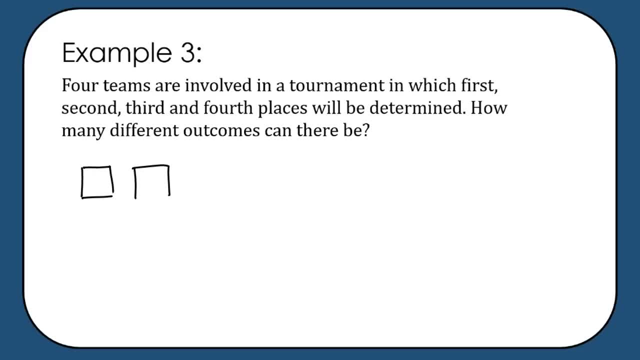 of use a pigeonholing kind of technique. Think about the different positions that are available in the problem. So here we have four different positions: First, second, third and fourth. Now we need someone to come first and someone to come second and someone to come third, and 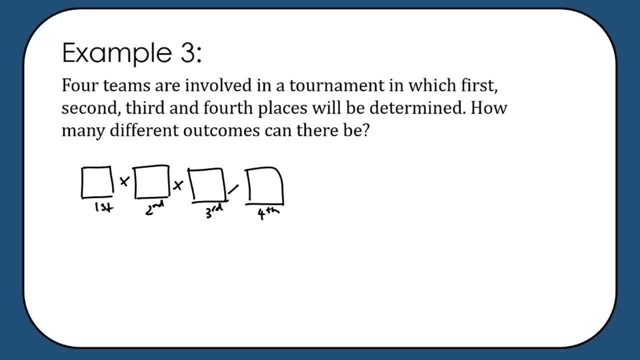 someone to come fourth. So we're going to multiply together the options for each of those. So we want to think about: okay, how many possibilities are there for someone to come first? There are four teams in the tournament. Any one of those four teams theoretically could. 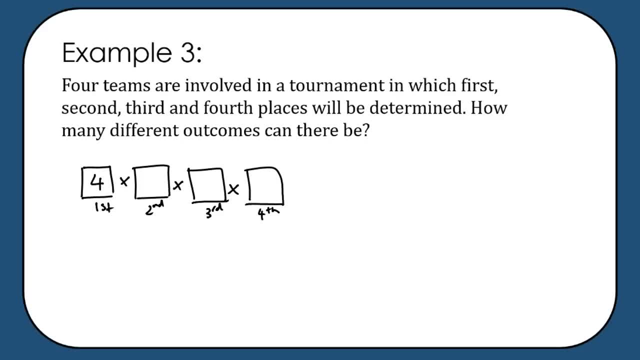 come first. Then we think: okay, well, how many teams could come second? Now, given that someone's already come first, there's now only three teams left that could come second, And we continue that. So there's two teams remaining that could come third and therefore the fourth position. 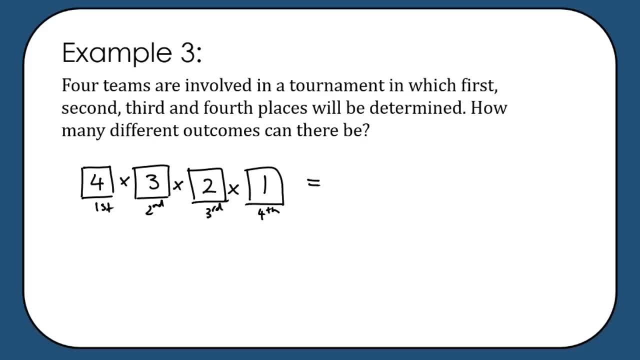 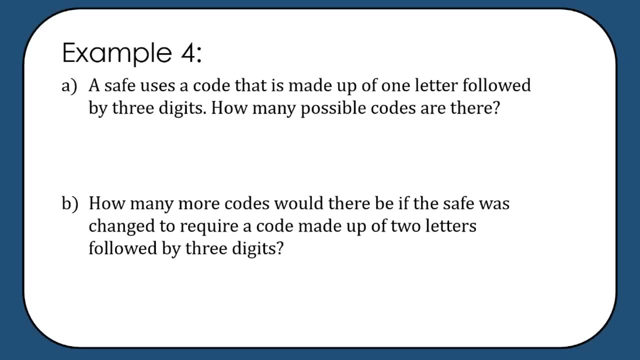 is filled once the third position is filled. And so four times, three times, two times one is 24 different ways that the four teams could finish in the tournament. Okay, a safe uses a code that is made up of one letter followed by three digits. How many? 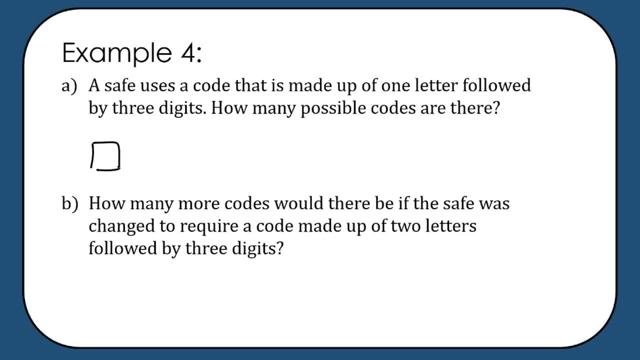 possible codes are there, Okay. so again, I've got sort of four positions. I'm going to go through them one by one. So I've got four options I need to fill. I need to fill all four of those. So this is the problem with- and I'm not filling the first digit or the third digit, I'm filling 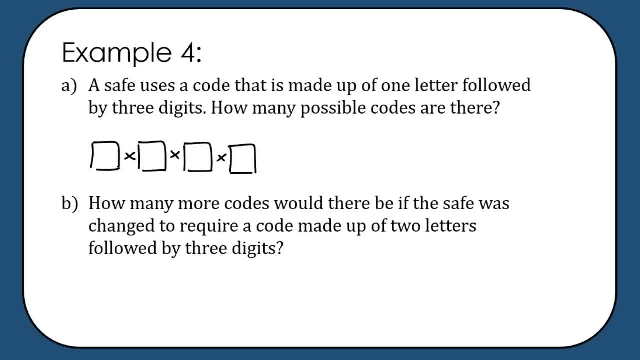 first digit, second digit, third digit and fourth digit. So this one needs to be a letter, The first two need to be a letter. Oh, no, sorry. The first one needs to be a letter and then the remaining three need to be a number, So made up of one letter followed by three digits. So then we want. 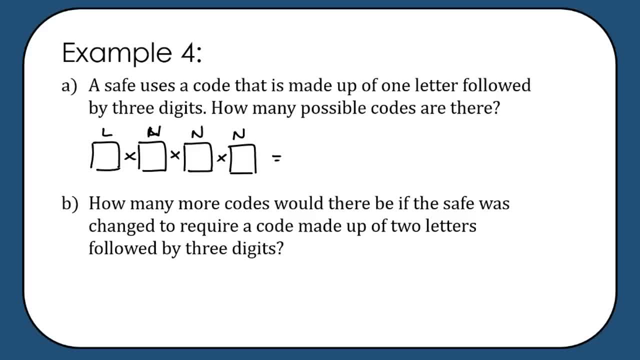 to think about well, how many options are there for each of these states, And then we're going to go through the stages. So the letter: obviously there are 26 letters in the alphabet, So 26 options for that. The numbers: the digits: there are 10 digits, zero to nine, So 10 different. 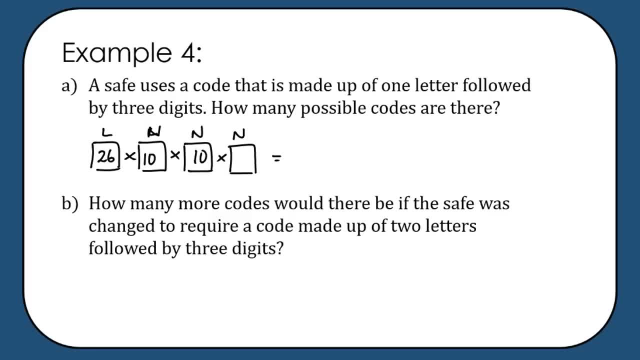 options that could go there: 10 different options for there and 10 different options for there. Given that there's nothing it says, we can't repeat the options. If it said that it had to be three different digits, then obviously it wouldn't be a letter. So 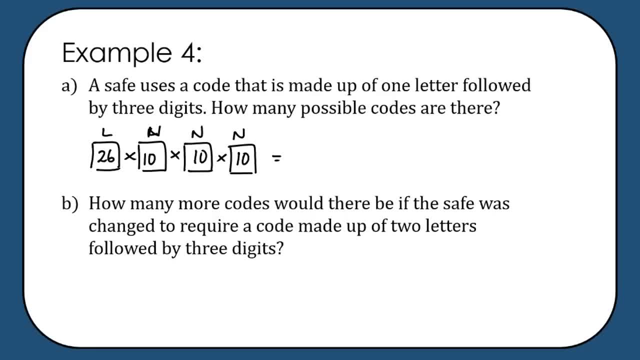 obviously there'd be 10 options for the first digit, only nine options remaining for the second digit and only eight options remaining for the third digit. Okay, so 26 times 10 times 10 times 10 is going to be 26,000 different safe codes. How many more codes would there? 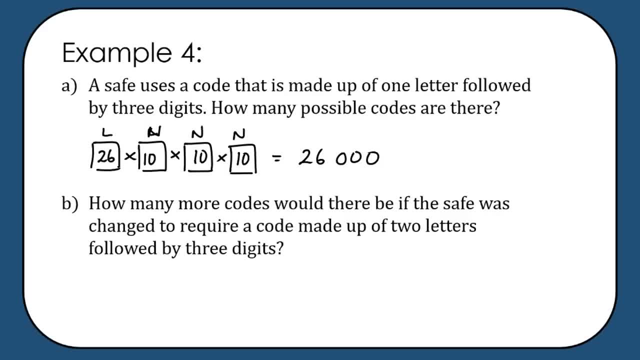 be if the safe was changed to require a code made up of two letters followed by three digits. So obviously this time we've got five positions in our code. We're going to be multiplying something in each of those positions, So it's an AND problem: 26 letters for the first.